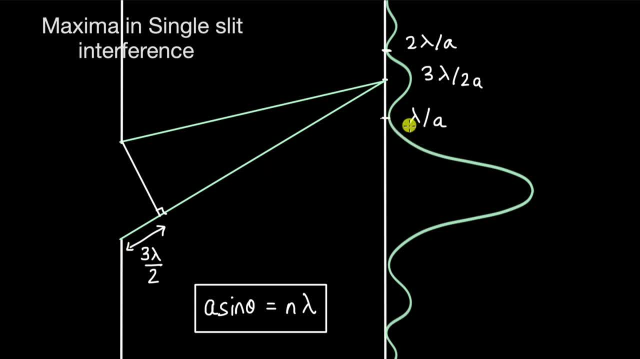 top source and the bottom most source was lambda for the first minima. for the second minima it is 2 lambda. So for the first maxima it should be 3 lambda by 2. We are checking if that, that really makes sense, if that's right. And I'm calling these sources because in a single slit all of the points. 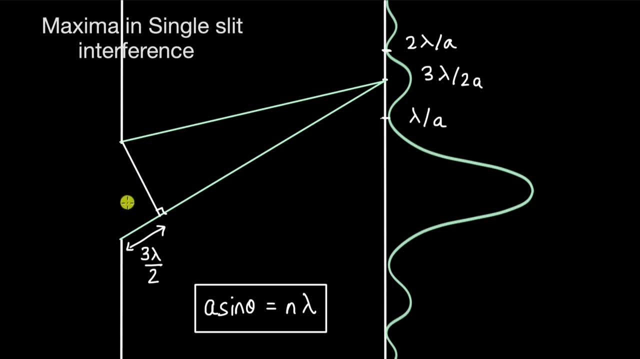 all of the points in the slit. they act as secondary sources, as per Huygens principle. They then interfere and create this pattern. Okay, so the part difference between the top most source and the bottom of source is 3 lambda by 2. So they should destructively interfere, But the top most source will also destructively interfere. 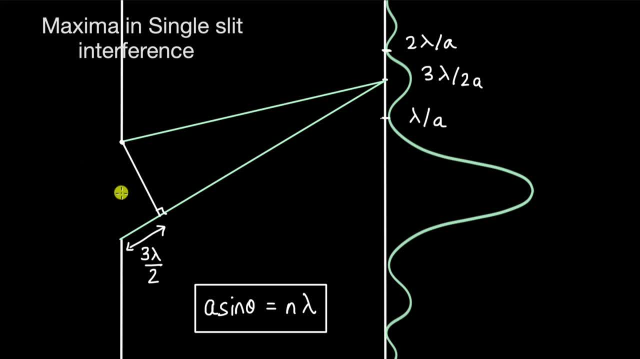 with a source with which its part difference is lambda by 2. Here the part difference is 3 lambda by 2.. But the top most source will destructively interfere even before, even with a source that is in between, because the part difference with that source will be lambda by 2.. You will come across. 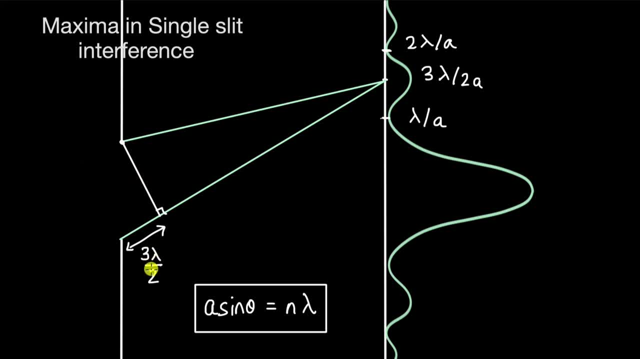 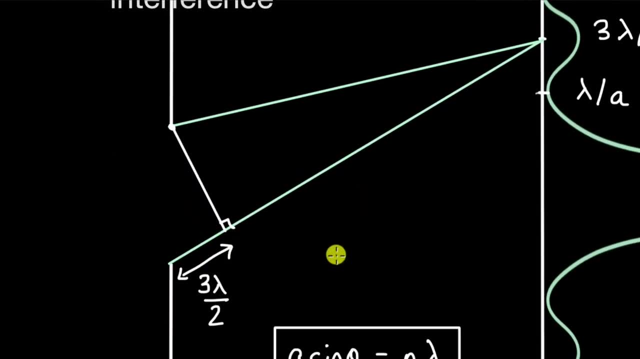 0.5 lambda, right lambda by 2 before reaching 1.5 lambda. So let's try and find where that source could be. We know that for this case we can write this as a sine theta: The part difference. a sine theta is 3 lambda by 2.. a sine theta is 3 lambda by 2.. Now if we divide both the sides by 3, if we 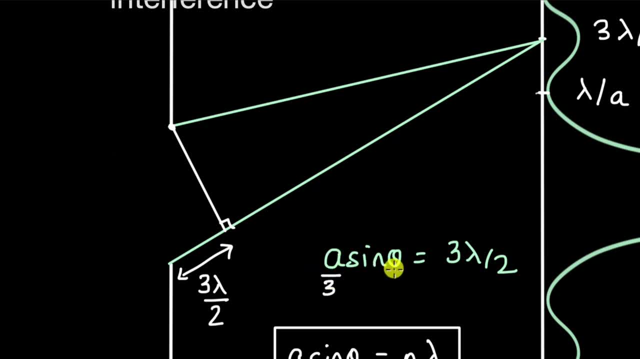 do that? if we do that, this becomes a by 3 sine theta, and this will be then equal to 3, will get equal to lambda by 2.. So what this tells us really is that all the sources that are a by 3 distance apart from each other, all the sources that are a by 3 distance apart from each other, the vertical. 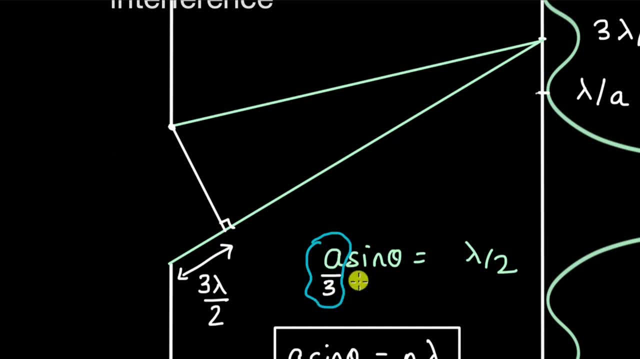 distance of a by 3 from each other, they will have a path difference of lambda by 2.. And if they have a part difference of lambda by 2, they should destructively interfere. So let's divide this, let's divide this whole a, this big a, into three smaller a's. When we do this we get a path difference. 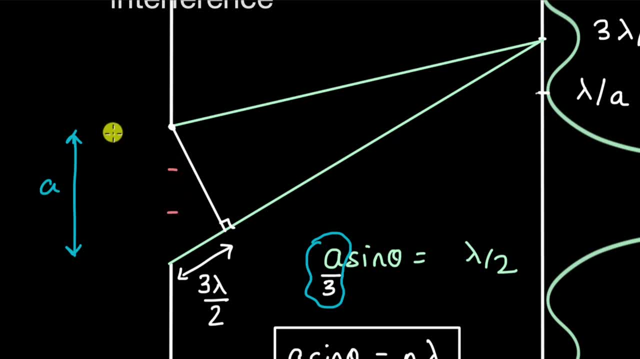 that this is, let's say, like this: So this right here is a by 3, this is a by 3, this is a by 3.. So the top most point will destructively interfere at a point source over here, because the part difference between them, the part difference between them that will be, that will be lambda by 2.. This distance, 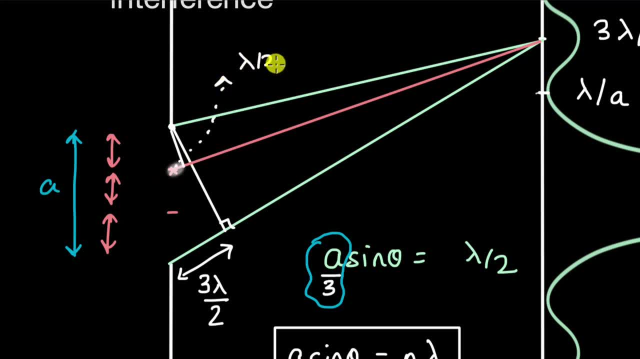 right here, this distance, this will be lambda by 2.. But this is not true for just these two sources. let's say, over here, this source and and some source that is in the middle section, maybe over here this. this source is, let's say, in the middle of the top section and this source is in the middle. 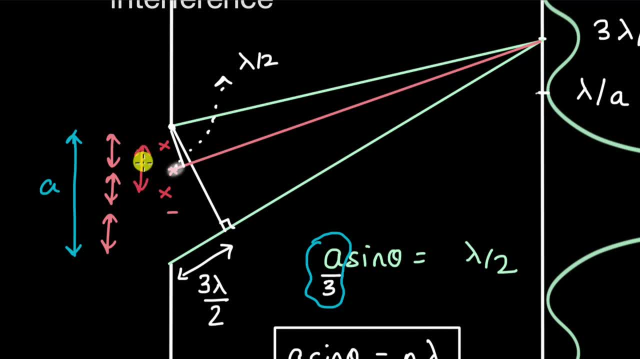 of the middle section. Even the distance between them will be a by 3. This distance is also a by 3. So that means that means that even these two sources, even these two sources, the part difference between them, the part difference between them, will be lambda by 2. So this distance, the 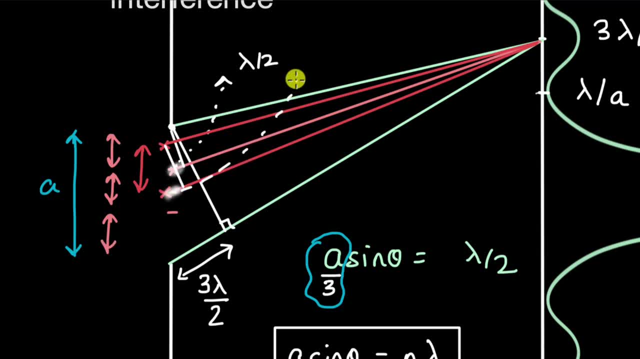 white part. this distance, it is lambda by two and turns out for all the points in the top section, in the top one-third part of the slate. all the sources in the top one-third part will have a source in the middle one-third part with which they will destructively interfere because a part difference between them. 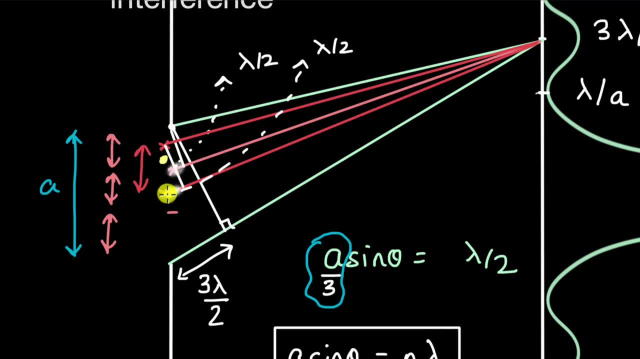 will be lambda by two. to pick, let's hit this point and this point right where the middle section ends. even even the distance between them is a by three and the part difference would be lambda by two. so turns out the top section. the top section cancels with the middle section. they destructively interfere with each. 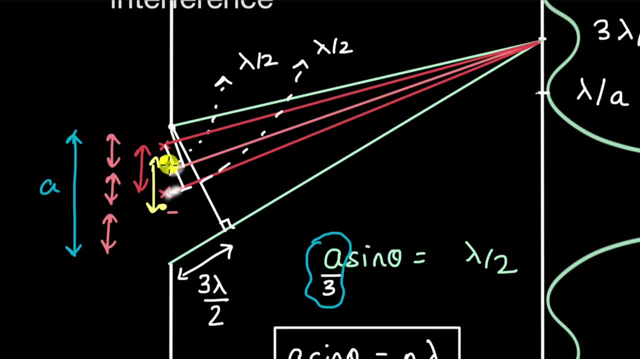 other. so the top two-thirds of the slate, the top two sections. they do not contribute anything. so if there is a maxima over here, it's not coming from these two parts of the slate. but no two sources are destructively interfering within the last one by third part of the slate, only the only. this. 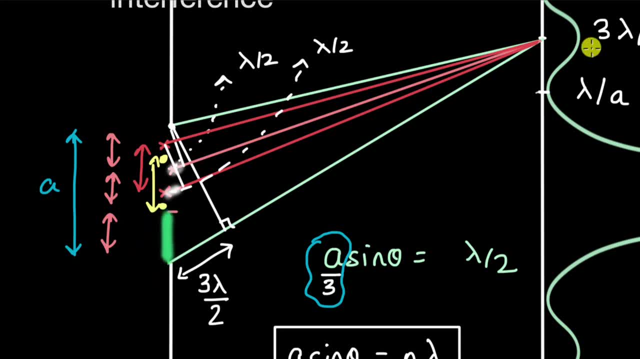 part of the slate, only this one-third of the slate contributes to the intensity at a point between the two minimas. so only this part of the slate leads to a maxima between the two minimas and clearly this is much weaker than the central maximum, because at the central maximum the entire slate contributed. 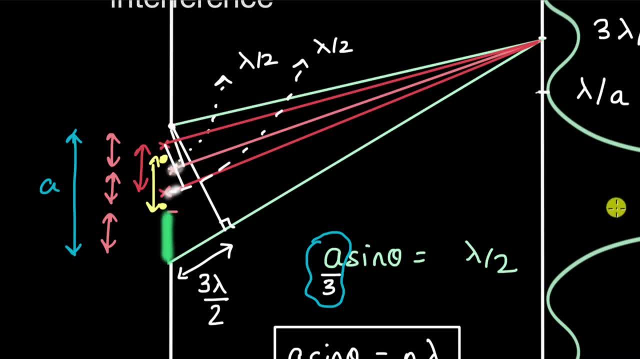 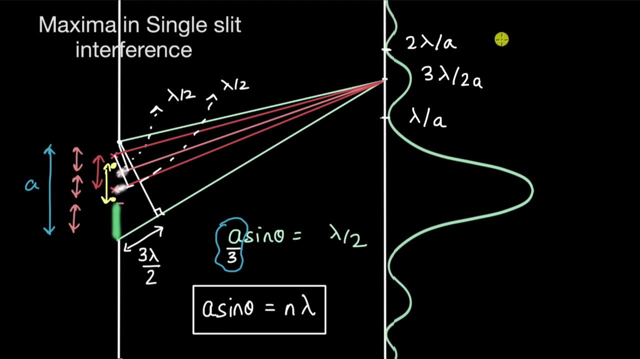 nothing got cancelled from each other. they all constructively interfered. here only one-third of the slate contributes. in phase the intensity is much less and we can say: we can say that maxima, that maxima are formed when the part difference, when the part difference is this is equal to: 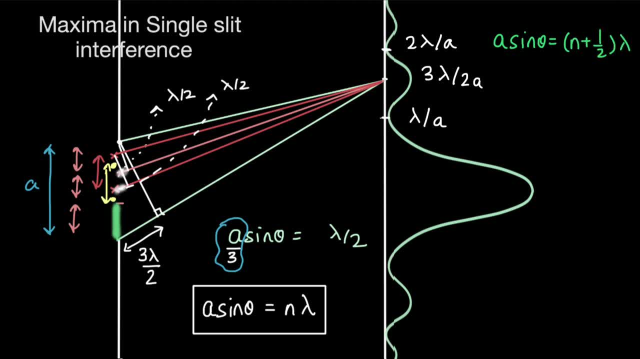 n plus 1 by 2 into lambda. so when n is equals to 1, a sine theta, this equals 3 lambda by 2 and there will be a maxima that with the first maxima, when n is equals to 2, you will get. you will get this maxima right here, but why does the 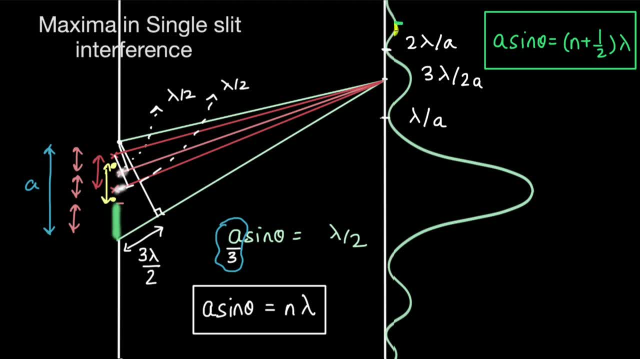 peak. why does the peak decrease? what is the intensity of the maxima decrease as you go further away from the center. when we were looking at the first maxima, that was the angular position, was 3 lambda by 2a. we divided the slate into three parts. if we look at the second, 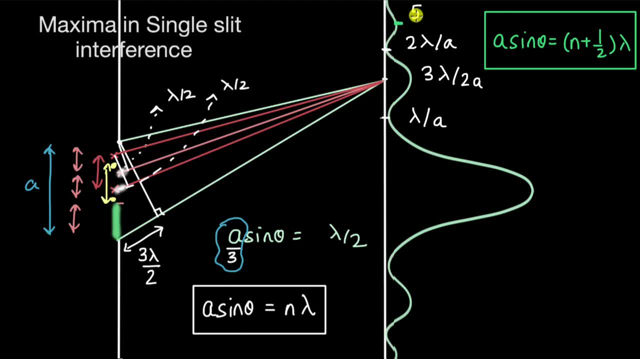 maxima. the angular position here would be: this would be 5 lambda by 2a. so here we will actually divide the slate into five parts. let's see how that would look like. so let's say: here we have, here we have a slate and we divide it in five parts. we divide it, we divide it into five parts. 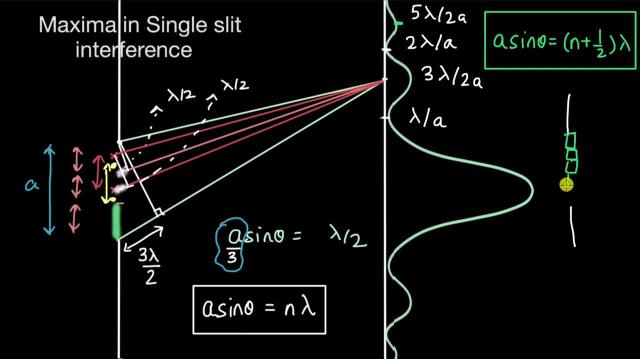 this is one, this is two, three, four and five. so in this case what happens is all the sources in the top, in the top section of the slate, destructively interfere with all the sources in this part of the slate, because the part difference between them remains to be as lambda by 2, and we can also see that. 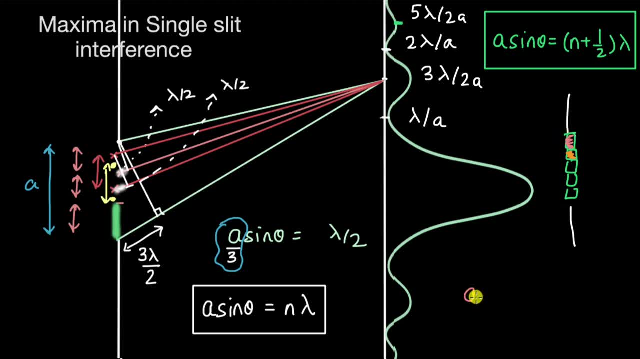 mathematically, initially, in the top most source and the bottom of source, we could have written a sin theta equal to 5 lambda by 2. but now, when we divide it, the slit into five parts, this becomes a by five. a by five and this five goes away. so any two sources. 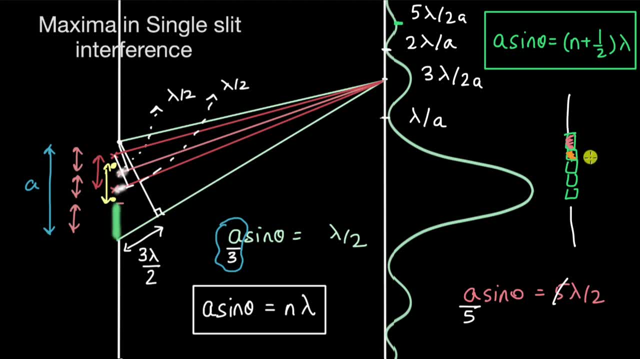 which are a by five distance apart, they will destructively interfere and that happens with any source in the top part and any source in this part, in the yellow part of the slit, and similarly that happens with with all the sources in this part of the slit and any source, any source in. 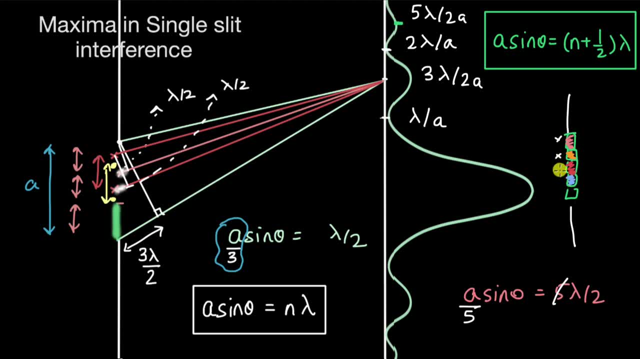 let's say, let's say this part of the slit. even between them, the distance remains to be as a by five, which comes out to a part difference of lambda by two, and a destructive interference that only leaves the bottom, most part of the slit, only this part of the slit, and here we see only